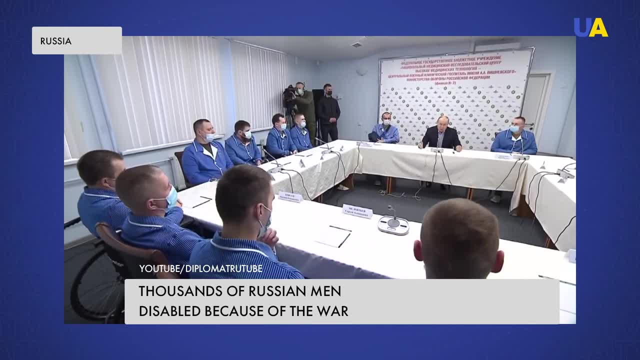 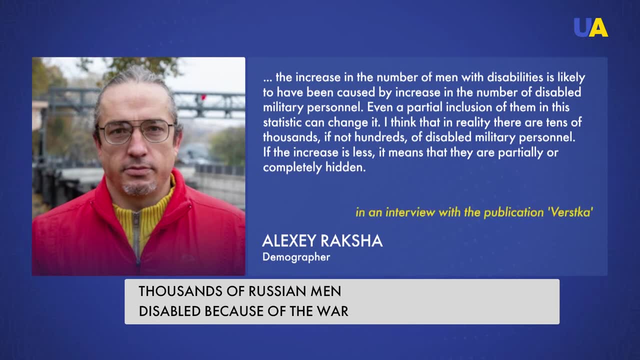 to 30 years. This is a record figure for the last eight years. The increase in the number of men with disabilities is likely to have been caused by increase in the number of disabled military personnel. Even a partial inclusion of them in this statistic can change it. I think that in 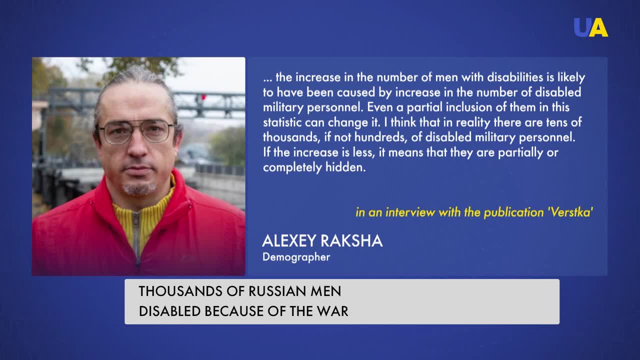 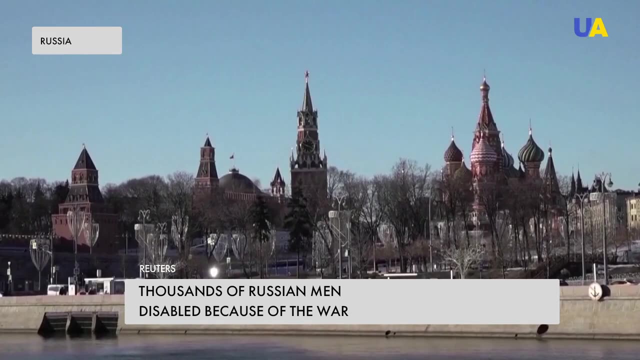 reality, there are tens of thousands, if not hundreds, of disabled military personnel. If the increase is less, it means that they are partially or completely hidden. Alexey Raksha, demographer, in an interview with the publication Verstka, And the number of. 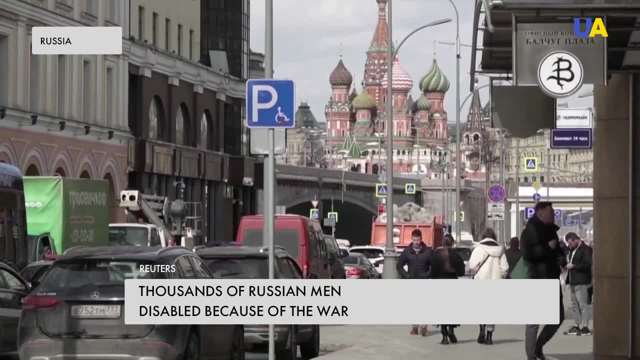 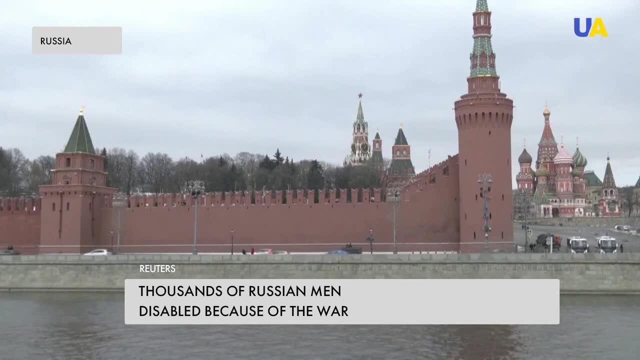 Russian men injured at the front will increase for as long as Russia continues to wage war against Ukraine. For the Federation's economy this is no small burden And at the same time, such dynamics will lead to an even greater shortage of labor force and will inevitably have a negative impact. 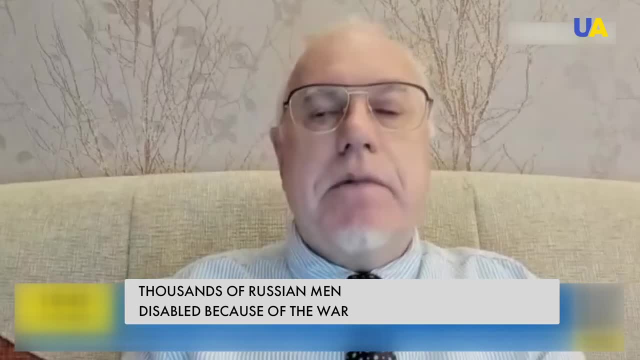 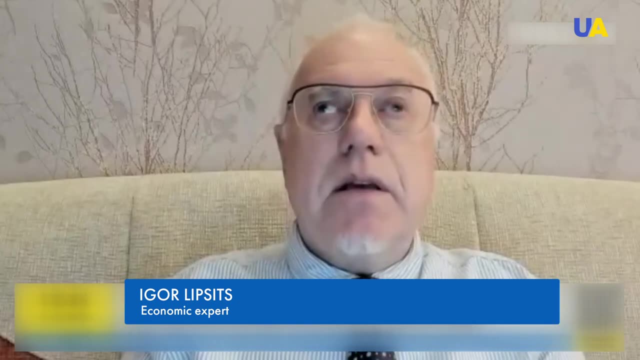 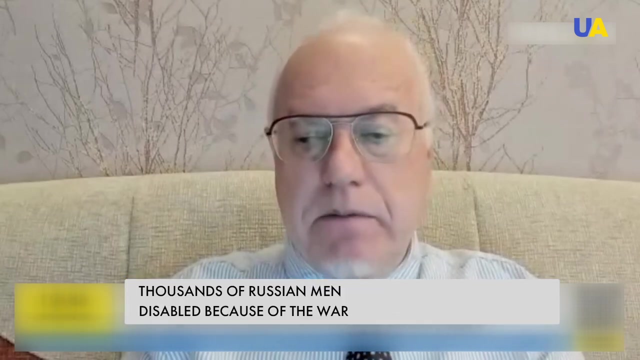 on the demographic situation In the wars of World War I and World War II, when Russia suffered huge human losses and this generally affected the dynamic, the population declined, But what happened in 2022-2023 is, of course, a catastrophic situation. 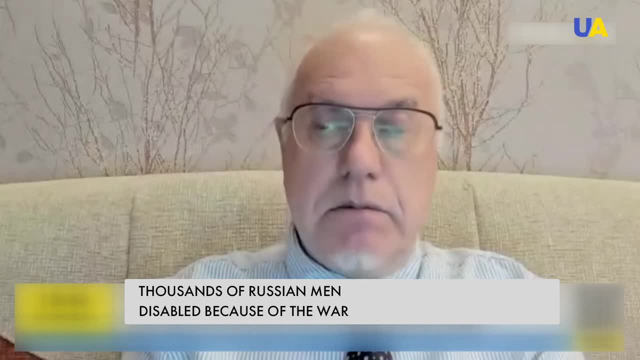 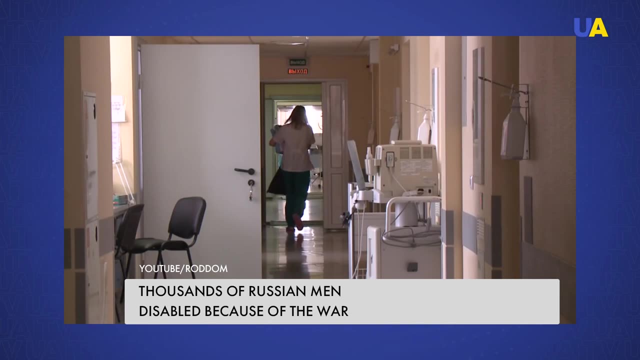 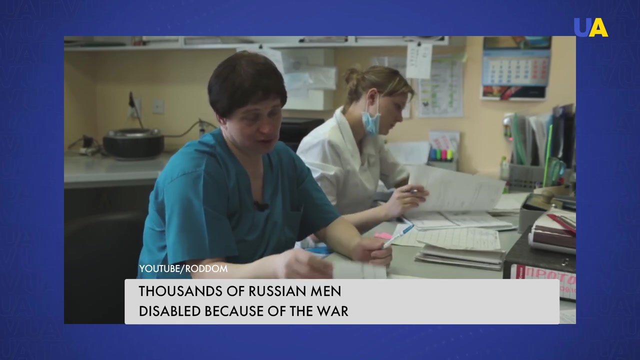 because at this point we lost hope of at least neutralizing the negative demographic trends In 2023,. according to official data, 1,200,000 citizens were born in Russia. this is the lowest figure since the collapse of the Soviet Union in 1991.. The demographers predict that 2024 will be the worst year of birth rates in Russia since the beginning of the 19th century. What is happening now? that people are dying, that many people are becoming disabled in Russia, that hundreds of thousands of people have left not wanting to fight. 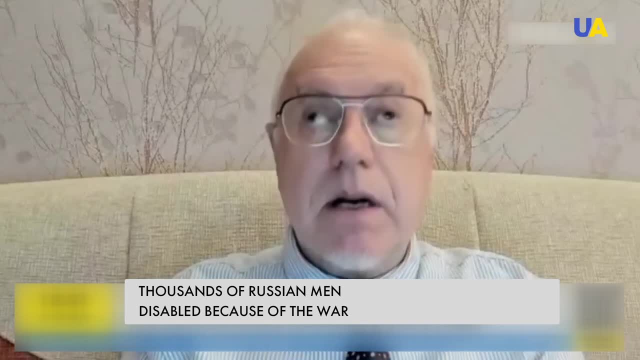 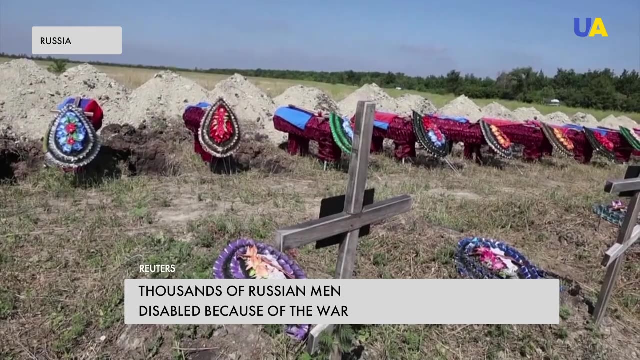 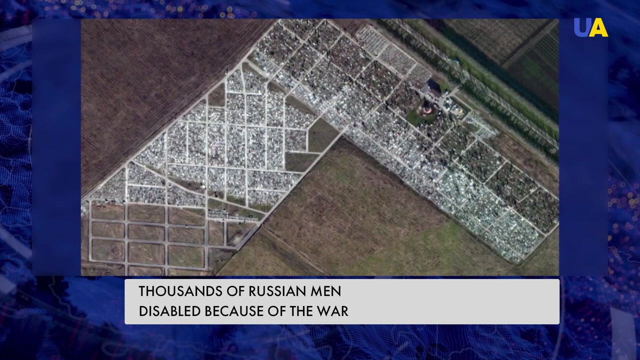 these are all dramatic things for demography. The number of burials in cemeteries associated with the Russian Defense Ministry and PMC has also increased sharply in the federation. The Telegraph reports In one section of the Tula cemetery alone, the number of graves quadrupled between October 2021 and April 2023. In the same 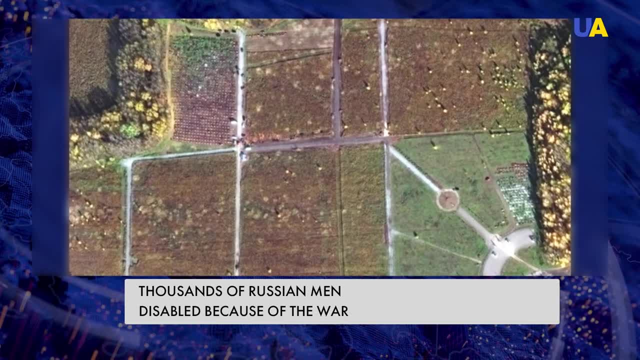 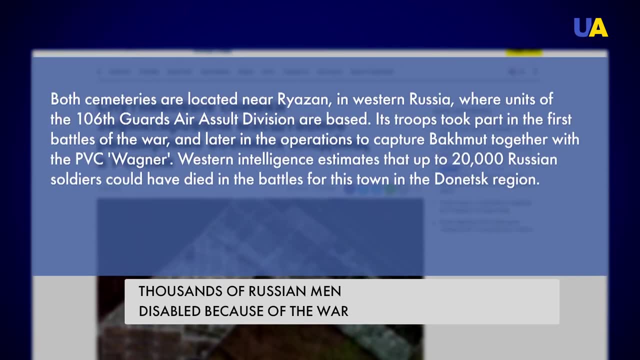 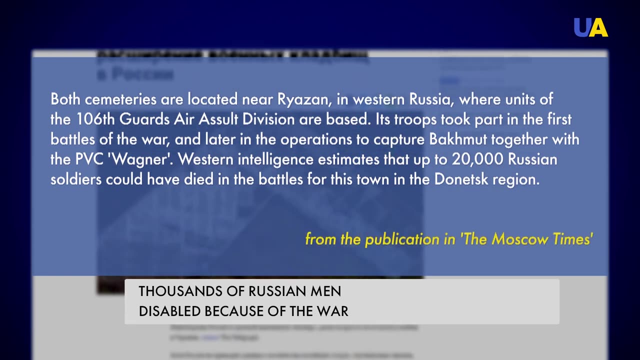 period of time, a brand new section appeared in the neighboring cemetery, which tripled in size. Both cemeteries are located near Ryazan in western Russia, where units of the 106-gallon Air Assault Division are based. Its troops took part in the first battles of the war and later.